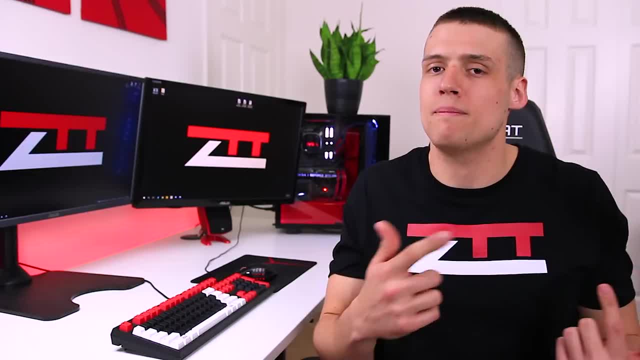 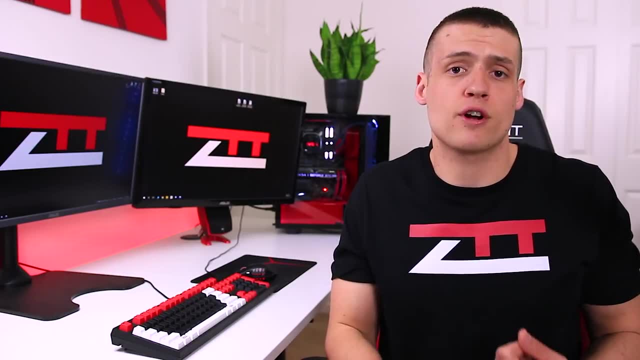 A stability test is something like AIDA64 or Prime95, where you just let your computer run it and you make sure that it doesn't get an error or crash. But a benchmark is something that you can have your computer run. that will give you a very consistent score and then you can use that score to compare it to other scores. 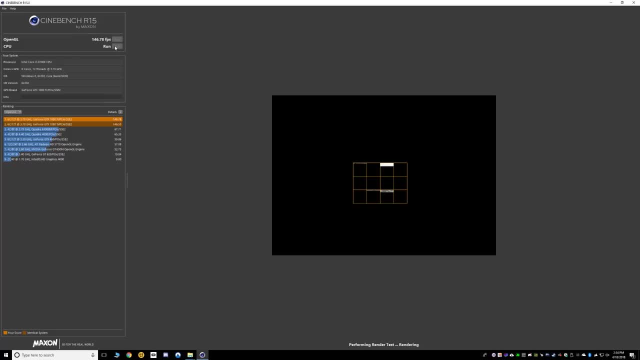 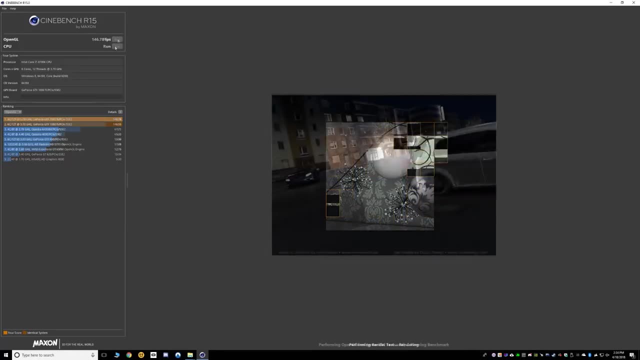 Some people get that confused. Alright, so the first benchmark on my list, which is in no particular order, is Cinebench, which you can download absolutely free from the link in the description. I'll put all the links down there. by the way. Cinebench is one of my favorites because, after it's installed, it requires zero setup, and 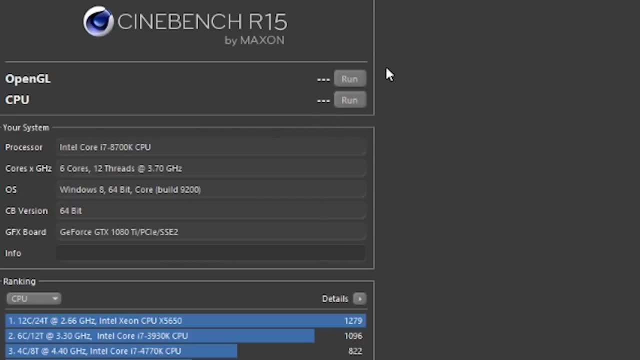 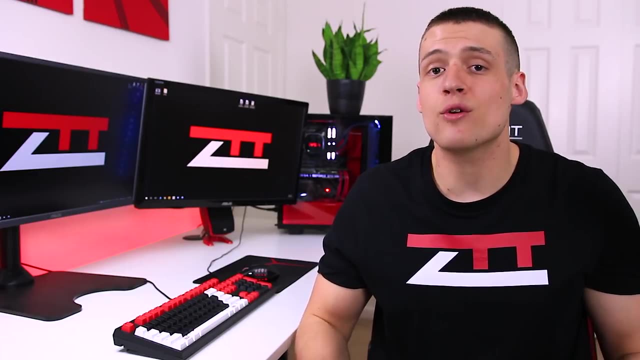 all you have to do is click run for either the CPU or the GPU test. I really really like Cinebench because there's no setup at the beginning, which means you don't have to change any settings and you can quickly see how your CPU is comparing. 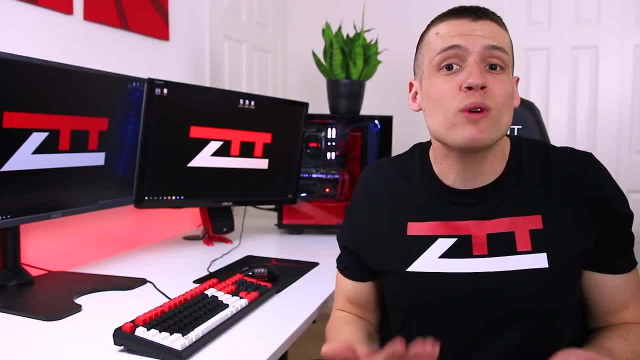 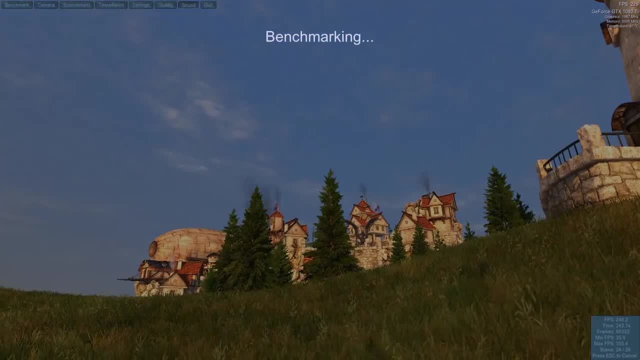 to other people with the exact same CPU. plus, you can really easily tell what kind of performance increase you get after overclocking. Moving on, our second benchmark on the list is the Heaven benchmark from Unigine, which has been around for almost 10 years now. 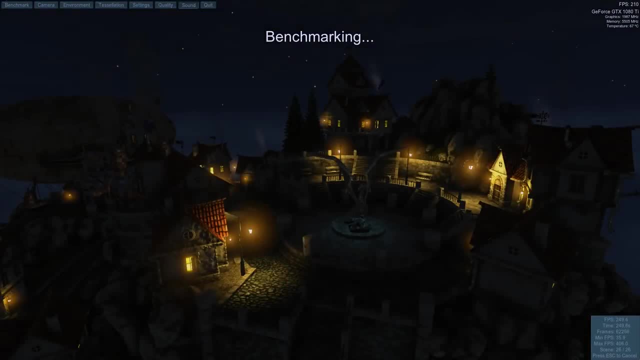 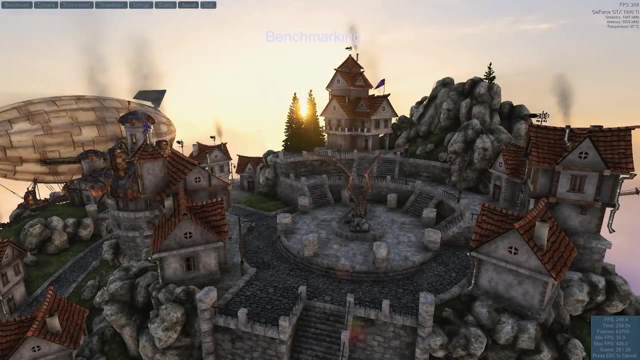 This is more of a GPU benchmark and it can also be used as a stability test. after overclocking. A lot of people just let the application run and make sure their GPU stays stable. but if you hit F9 on your keyboard, it'll start a 4 minute long benchmark and at the end of 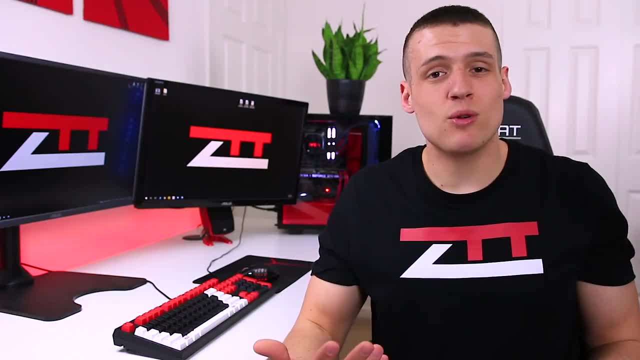 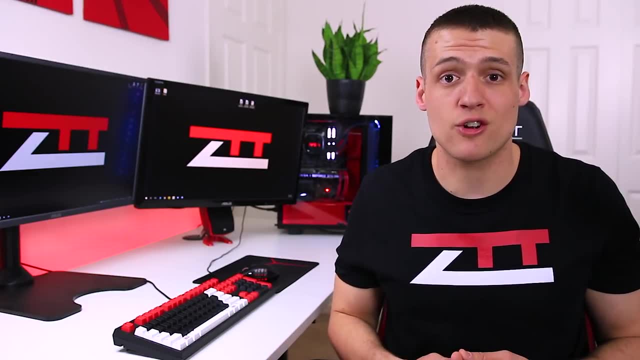 it, it'll give you a final FPS average and score. The thing I really don't like about Heaven is that there's a lot of settings to configure in the beginning, which just means if you're trying to test your overclock, you need to make sure that you're using the exact same settings every single time, and if you want, 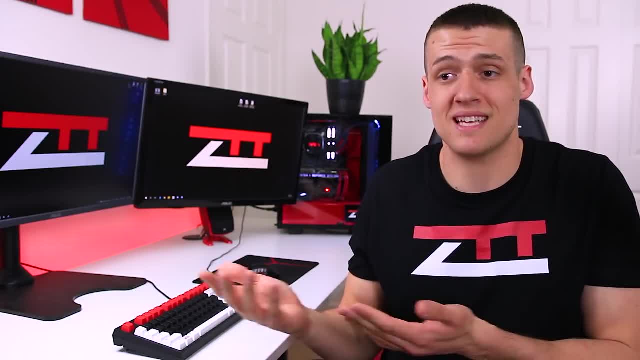 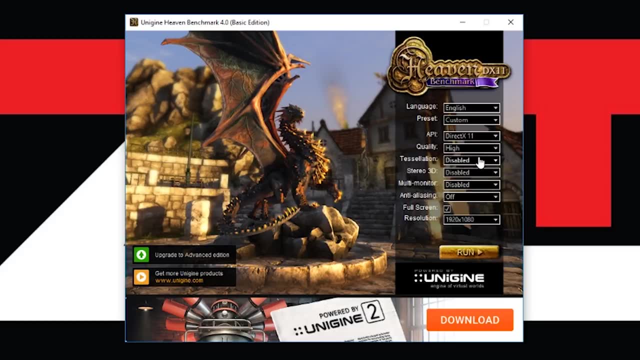 to compare your results online, you have to make sure that you're using the same settings that someone else did. Don't get me wrong, though. having flexibility is awesome. you just have to make sure that you're setting your API quality, anti-aliasing and all of those other settings the same way. 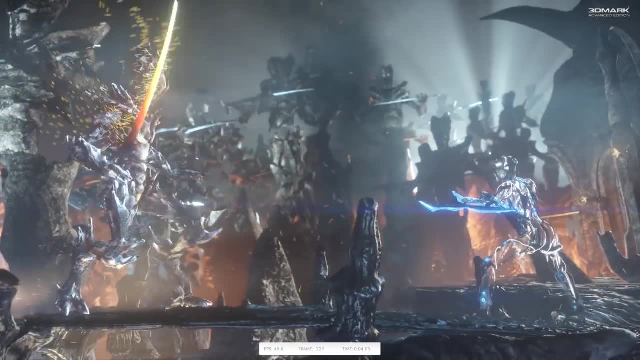 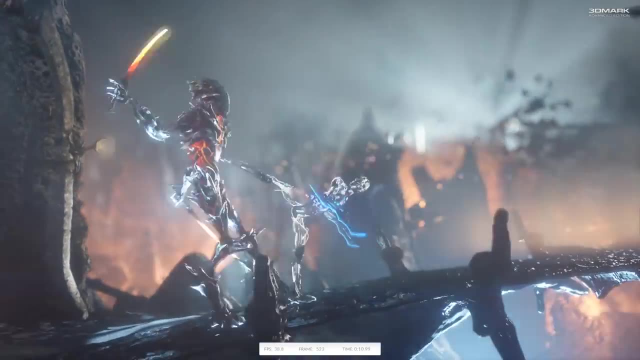 every time. that way you can get consistent results. Next up on our list is probably my favorite out of all of these synthetic benchmarks, and that's the famous 3DMark. You can download the 3DMark demo for free on Steam or from the link in the description. 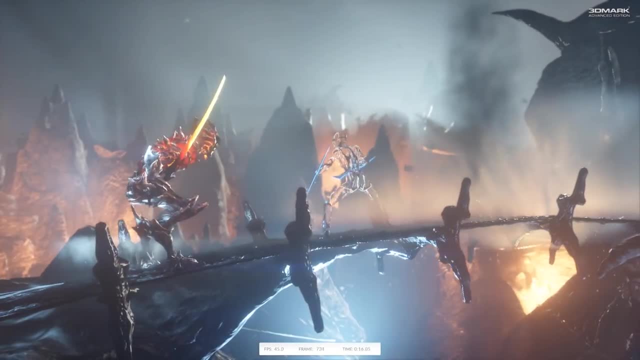 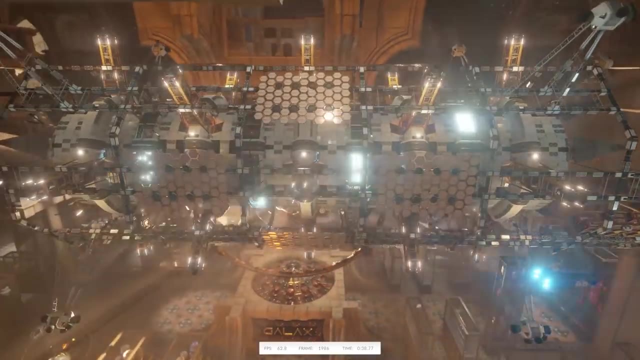 It's on our website and it'll let you run some of the benchmarks, but I do have the paid version here, which gives me access to some settings and more benchmarks. The recommended benchmark right now is Time Spy, which is a DirectX 12 benchmark just. 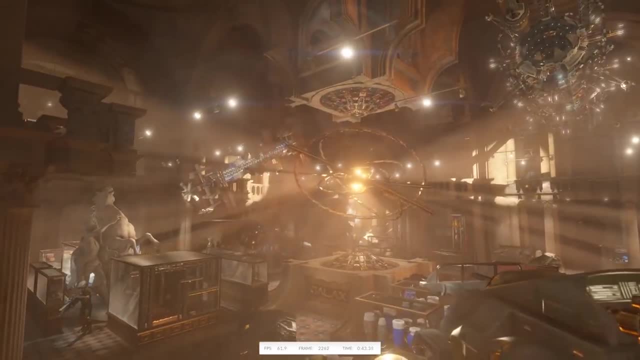 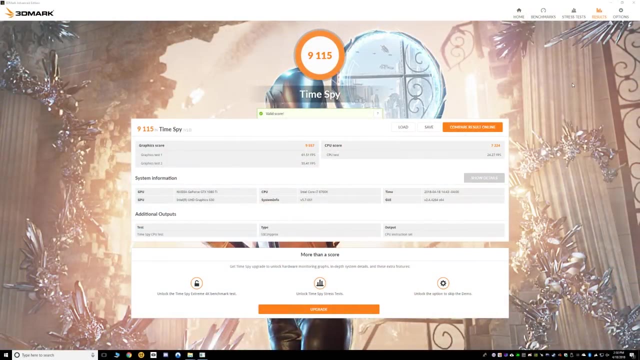 like the rest of these, it'll measure both your CPU and GPU. The other popular ones are the Fire Strikes. they even have an Extreme and Ultra version to test those super baller PCs. What I really like about the 3DMark benchmarks is that it breaks it down into multiple tests. 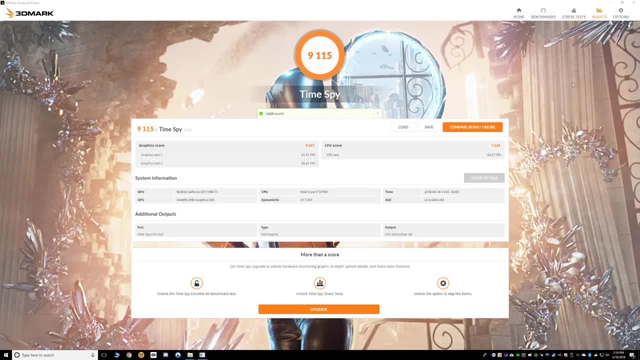 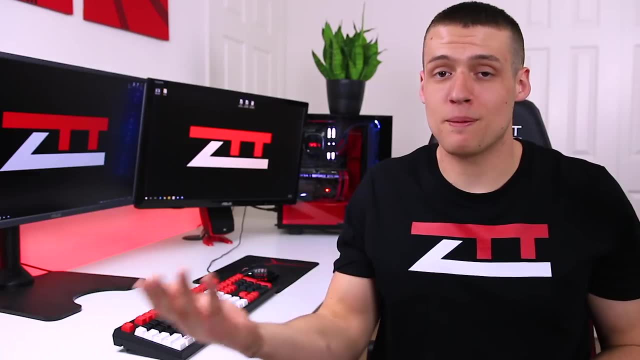 for the CPU and GPU, so you'll get a score for both, But then at the very end you'll also get a score for both. You'll also get a total system score, which is great to compare to others. You can then take that score and compare it to other people's PCs online, and I think 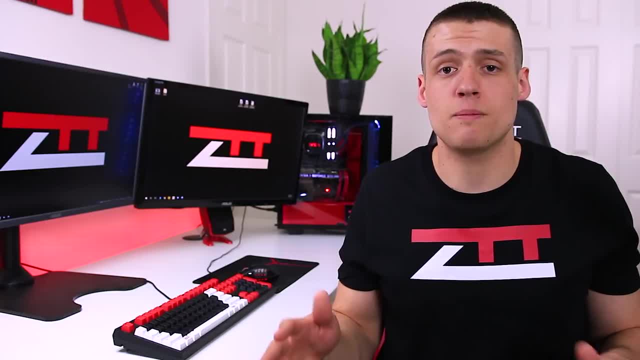 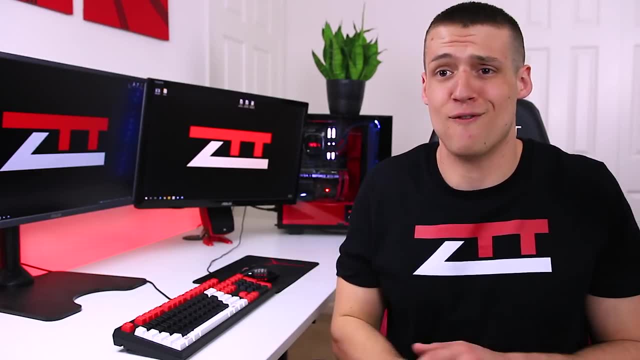 it's pretty cool because, like Cinebench, there are no settings to configure at the beginning, so everyone is on an even playing field. It's pretty cool to know that this PC behind me is within the top 1% of all gaming PCs in the entire world- well, at least PCs that have actually run the benchmark. 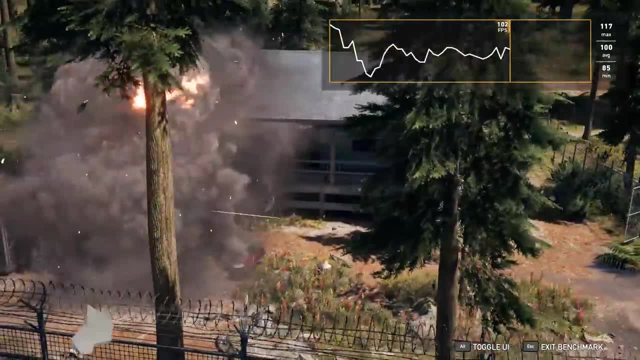 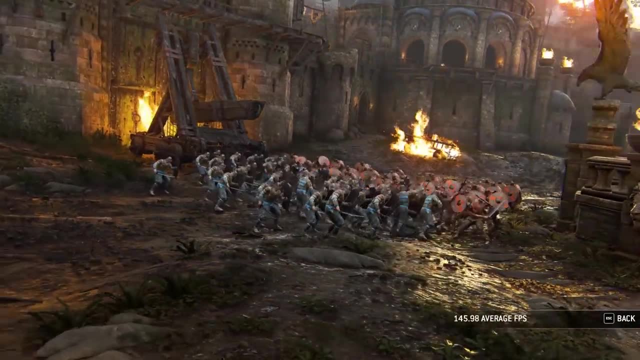 Moving towards the end of the list, the fourth benchmark that I really like is simply in-game benchmarks. There are a lot of games out there that include them. I definitely wish they did, but there are some good titles like Far Cry 5 and Assassin's Creed Origins that include awesome benchmarks. 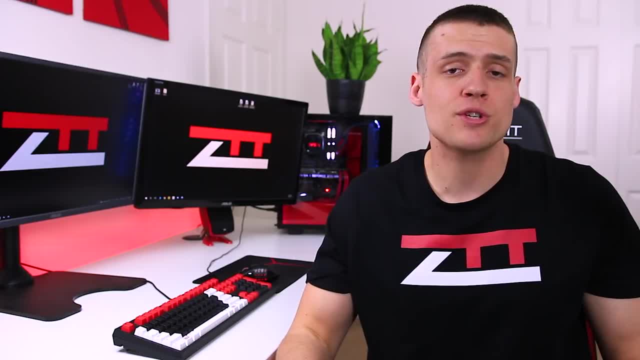 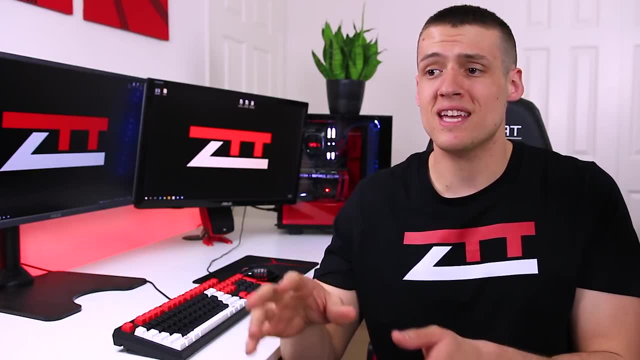 I really like using these because they're super simple to set up. all you do is adjust the video settings that you actually want to use in-game and click benchmark. but the one thing to note about these is that the performance you get in the benchmark doesn't. 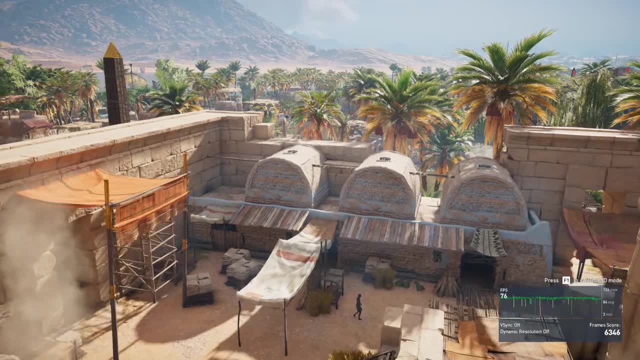 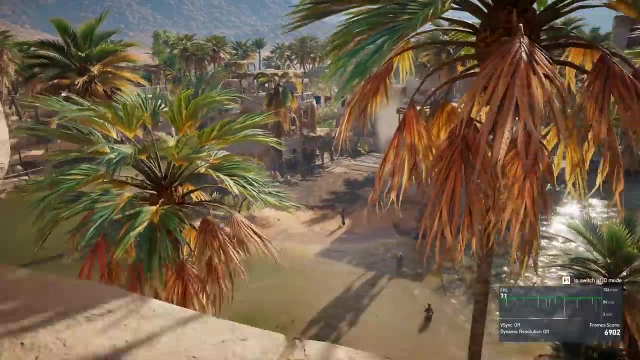 always represent the exact performance you'll get when actually running the game. For example, Assassin's Creed Origins is definitely a tough game to run, but the in-game benchmark is a good score than it is just to run the game. For some reason, different games have a benchmarking tool that's harder, so just be aware of. 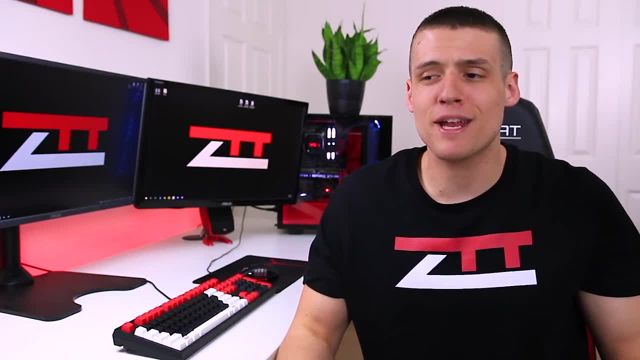 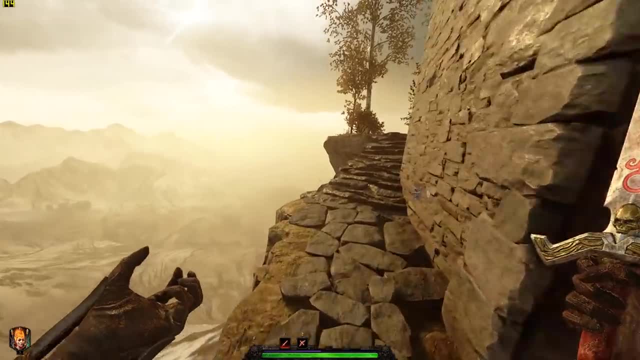 that And finally, my fifth benchmark is to just play any game that you want and run FRAPS. Just pick the game you want to test, set the in-game settings and just simply run the game. By using FRAPS, you can constantly monitor your FPS, like this in the upper left hand. 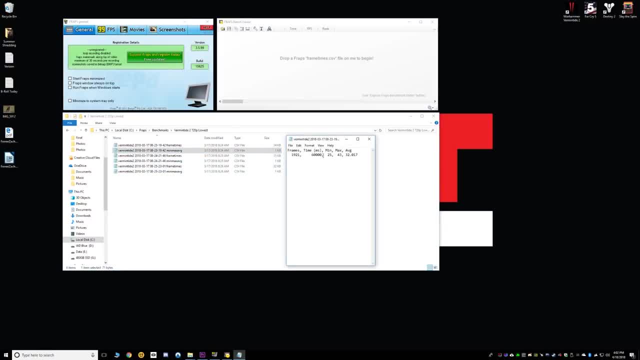 corner and you can export this data to text documents so you can see your min, max and average FPS settings. You can also combine this method with another free software like FRAPS. Drop the text file in there and FRAPS will then give you your average FPS: 1% and 0.1%. 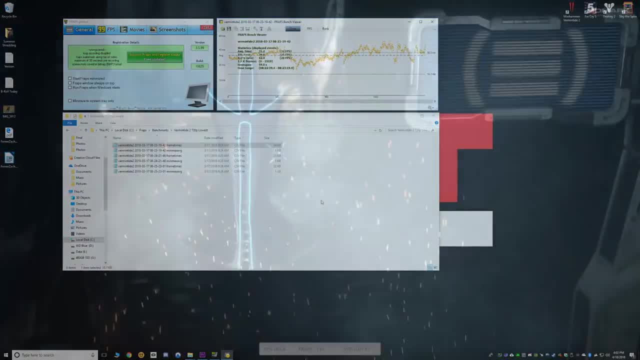 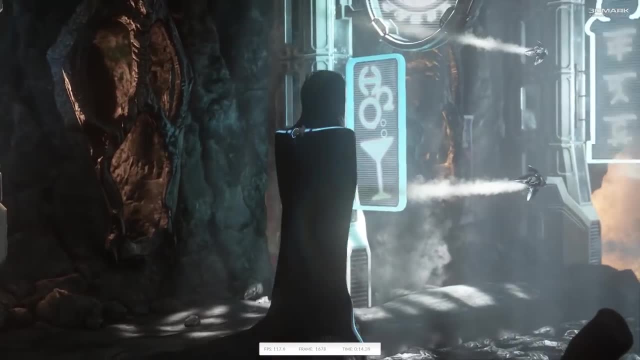 lows. This is actually exactly how I benchmark games for you guys. So, to recap, these are my personal top 5 ways to benchmark your PC, and there are certainly plenty of other options out there. I use Cinebench Heaven, 3DMark, in-game benchmarks and FRAPS on almost every single PC that I'm